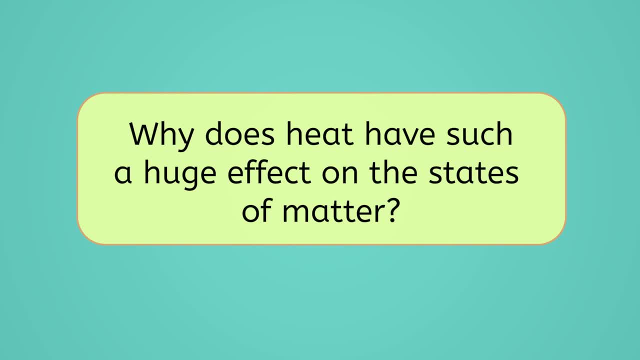 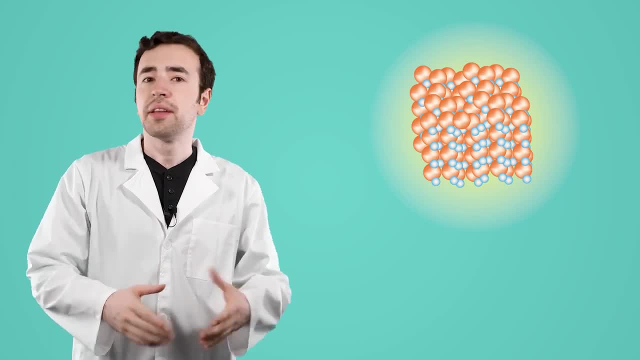 or addition of heat have such a huge effect on the states of matter? To answer this question, let's take a closer look at a solid. Now we know that the atoms of a solid are very closely packed together, and that's why it's called a solid. 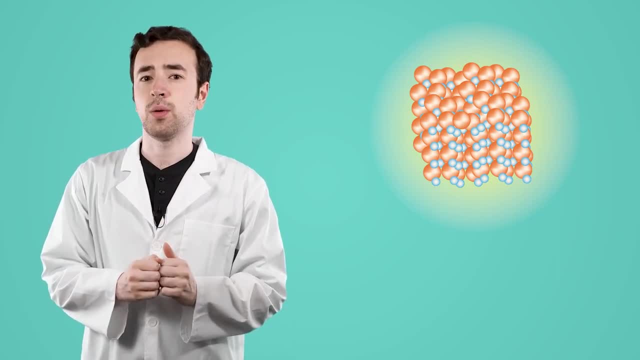 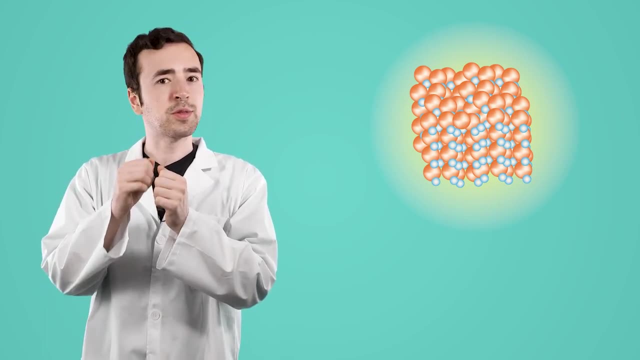 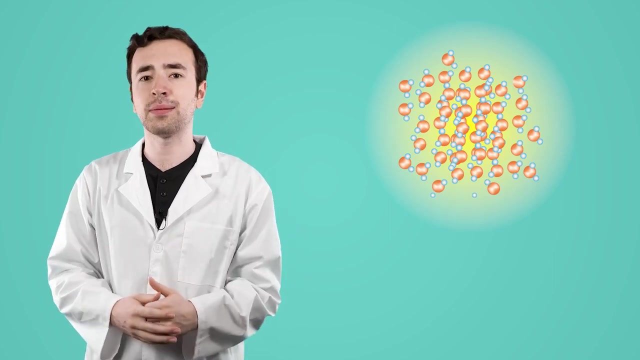 They're not really moving much. they're just kind of vibrating in place. Well, when we add heat to this, the atoms will start to speed up. This movement will cause them to start moving away from each other. What state of matter has atoms that are more separated and moving faster than a solid? 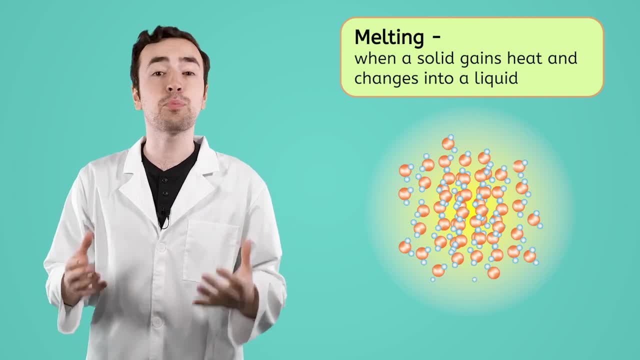 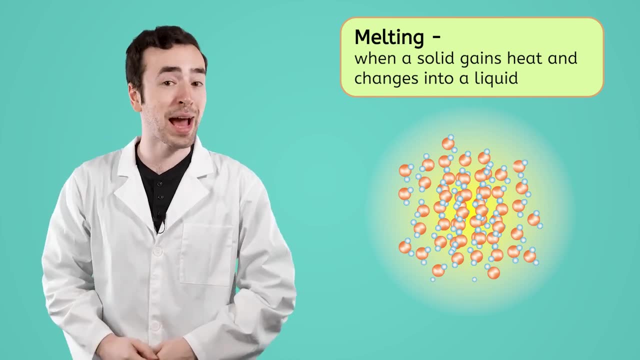 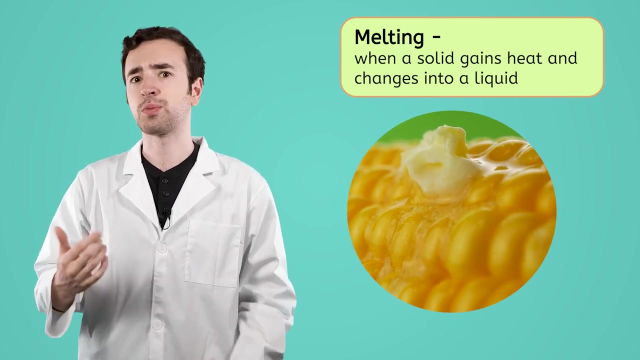 Yep, liquid Melting is the process of a solid gaining heat and then turning into a liquid. So that's what happened to my ice cream cone. It's also what happens when I put butter over hot food, And it's what happened to my snowman that I built when he met his first sunny day. 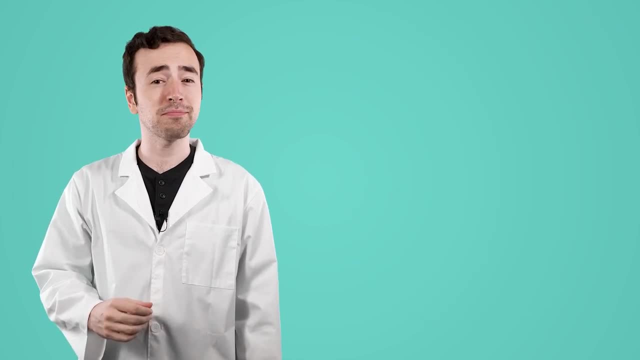 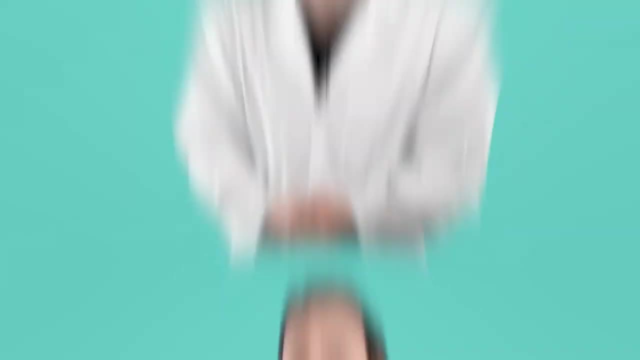 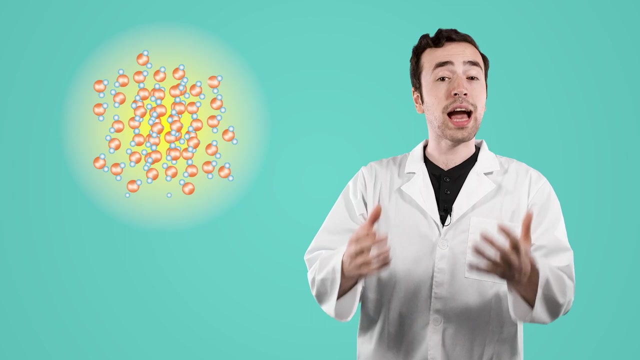 Now, can you think of any examples of melting? Pause the video here and jot down some of them in your guided notes. Alright, melting is cool and all, but What if we added more heat to a liquid? Well, the atoms in a liquid are moving and they're kind of sliding past each other. 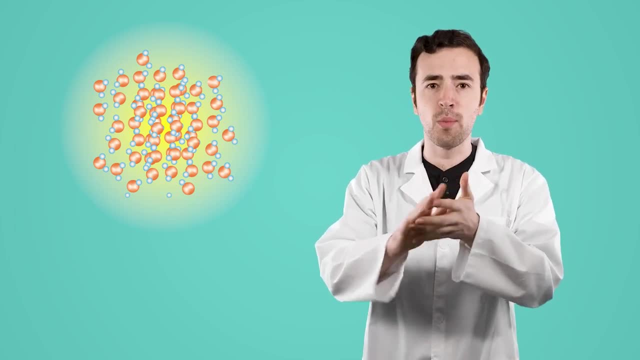 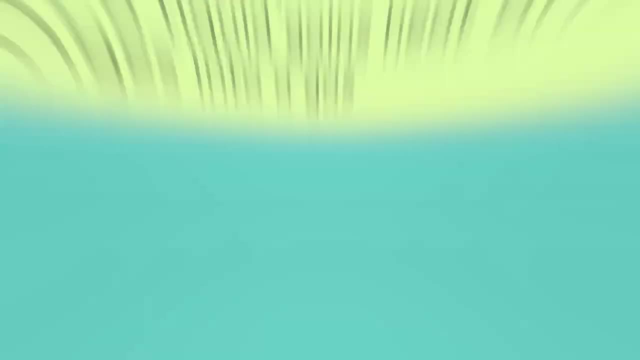 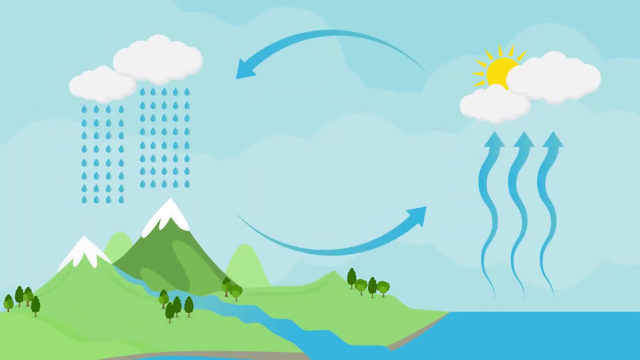 When we add more heat, the atoms speed up even more and this movement forces them apart. Now we have a gas. When a liquid gains heat and changes into a gas, it's called evaporation. If you've learned about the water cycle, you'll know that evaporation is happening. 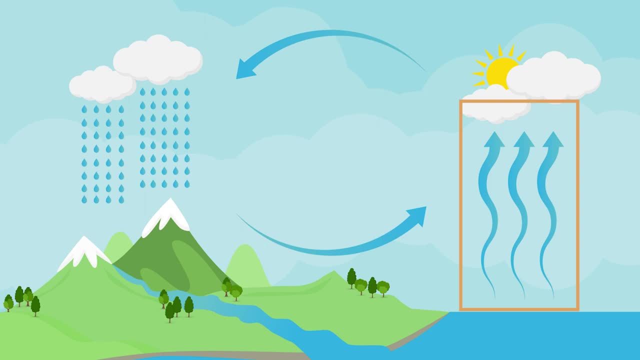 all the time. Water in our environment, changing from liquid to gas called water vapor, is an important part of that cycle. Evaporation is also what's happening when you hang up a towel to dry or when you let sweat dry from your own skin. 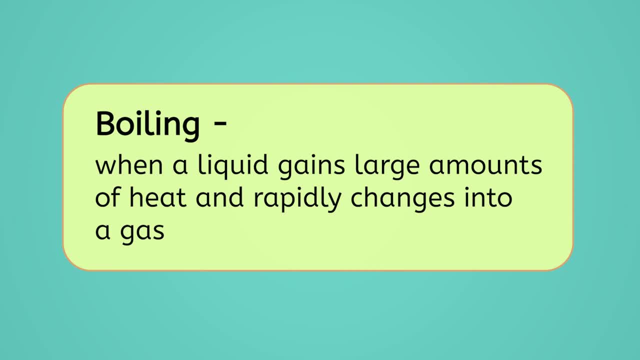 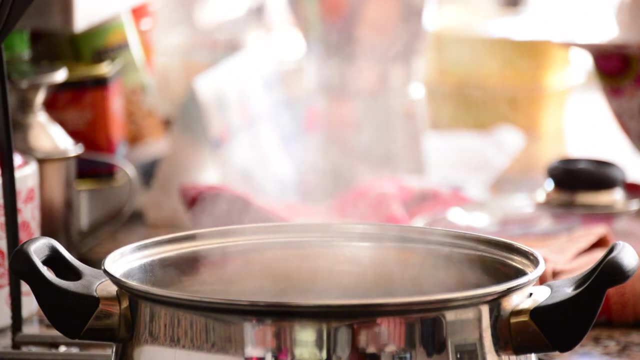 Another common way we see liquid changing to gas is through boiling or when a liquid gains large amounts of heat and rapidly changes into a gas. Think of the last time you saw a pot of water heating on the stove. You probably noticed steam rising from the pot. 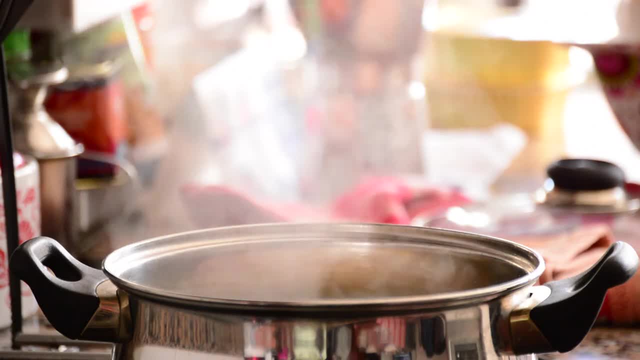 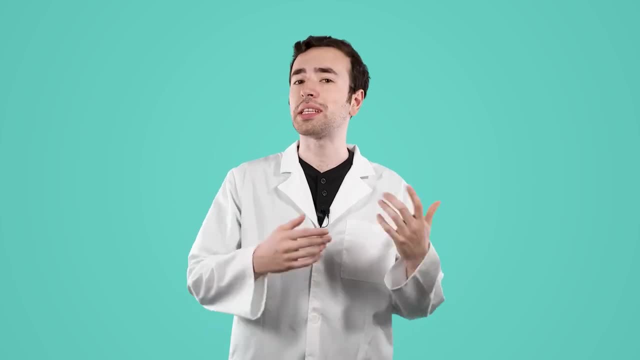 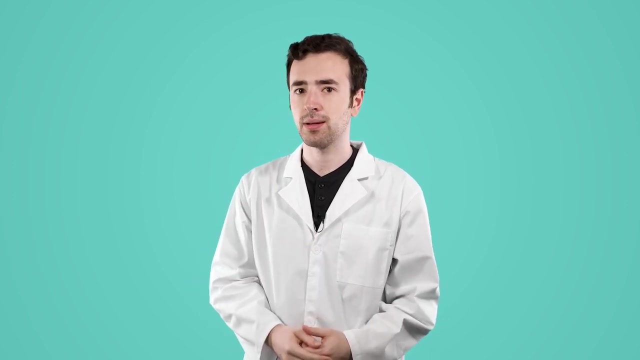 The heating water boiled and it changed state to water vapor that you see as steam. So Solids turn into liquids and liquids turn into gases. when we add heat, What do you think happens if we remove heat from something? Now notice how I'm not saying. what do you think happens when we add cold to something? because 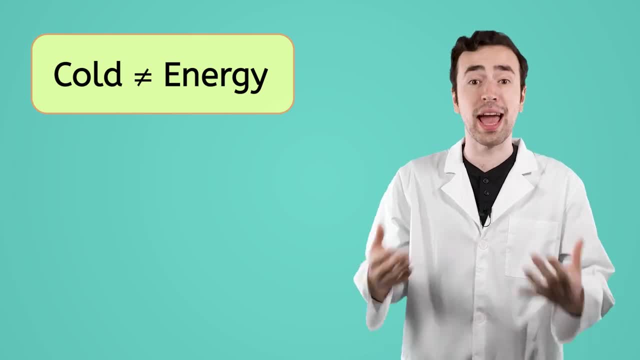 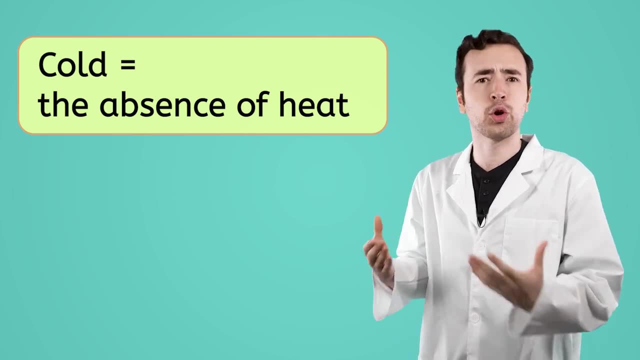 you actually can't do thatiah. some scream- Maybe I have to- when I just sayерх, Cold isn't a type of energy, it's just a way to describe the absence of heat. Even if you put something in the freezer, you're not adding cold to it, you're just. 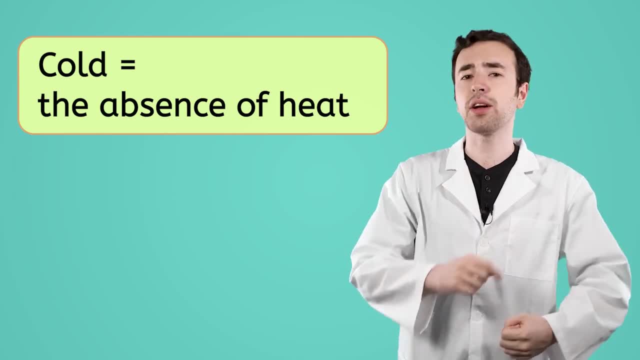 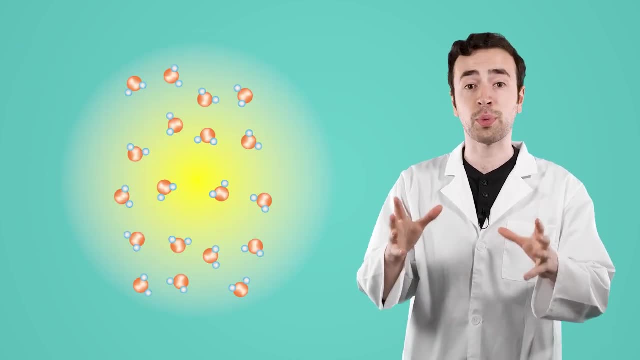 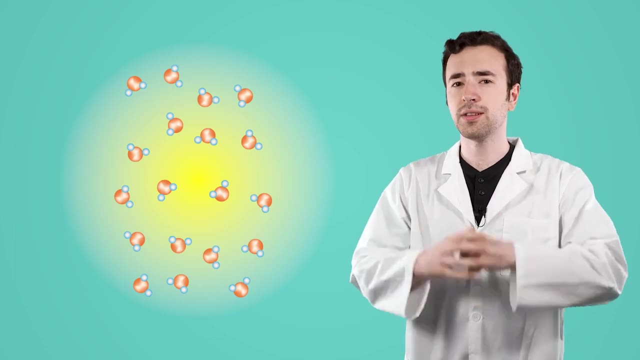 removing heat from it. Let's take a look at what happens to a gas when we remove heat from it. Remember, the atoms of a gas are all spread apart and they're moving around pretty fast. What do you think will happen when we remove heat from it? 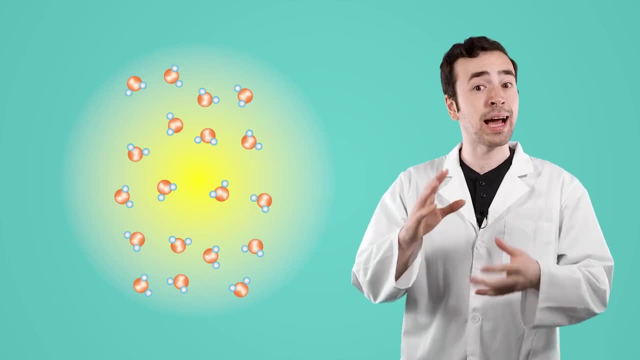 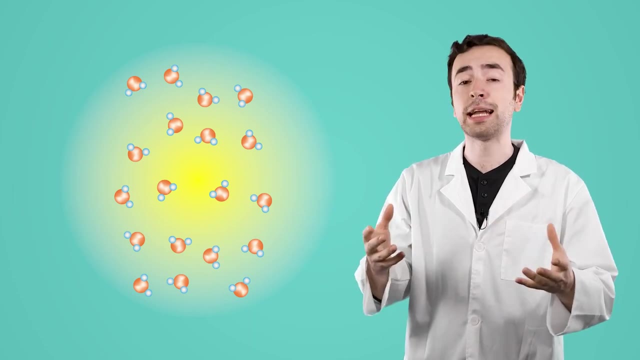 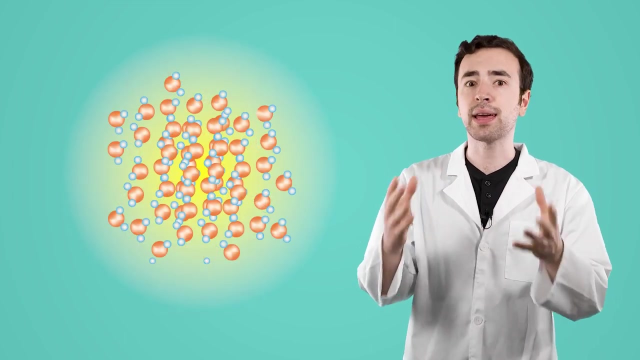 Well, when we add heat to something, the atoms speed up, and when we remove heat from something, the atoms will slow down. The atoms in the gas will start moving slower and slower and that will allow them to come closer together. The gas becomes a liquid. 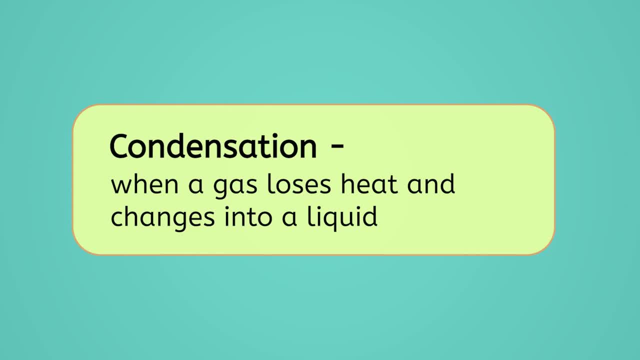 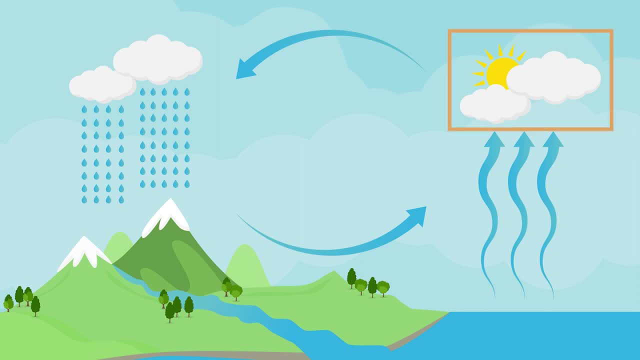 When a gas loses heat and changes into a liquid, it's called condensation. During the water cycle, water vapor condenses into clouds in the sky. Condensation is also the reason for water droplets on the outside of a cold drink or 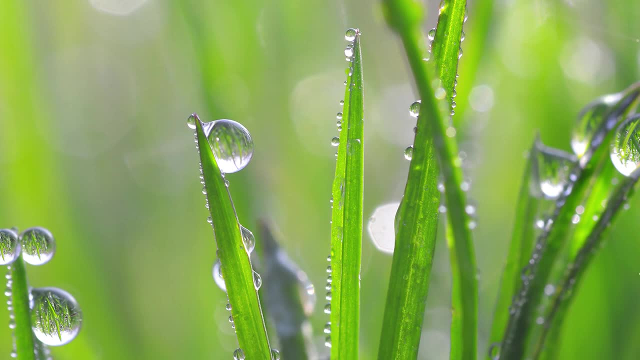 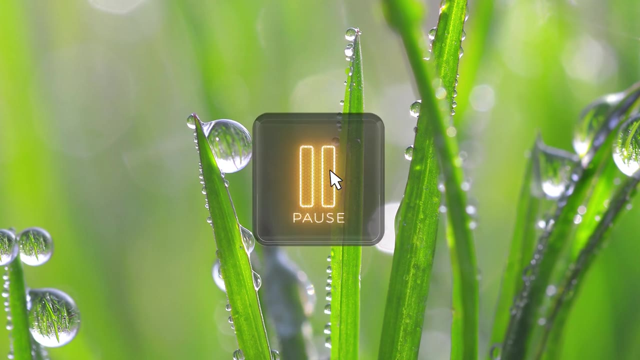 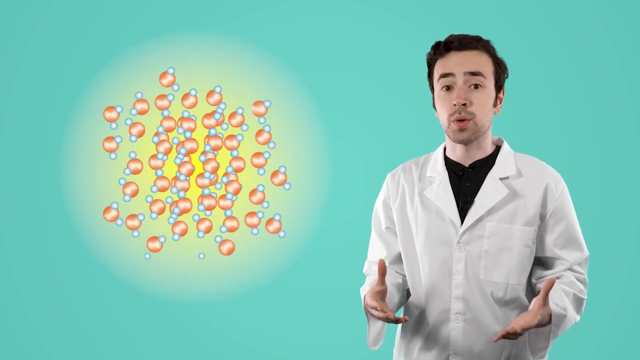 dew on the grass in the morning. Pause the video and write down an example of condensation that you've experienced in your guided notes. So what happens when a liquid continues to lose heat? Well, the atoms in a liquid are all loosely packed together and sliding past each other. 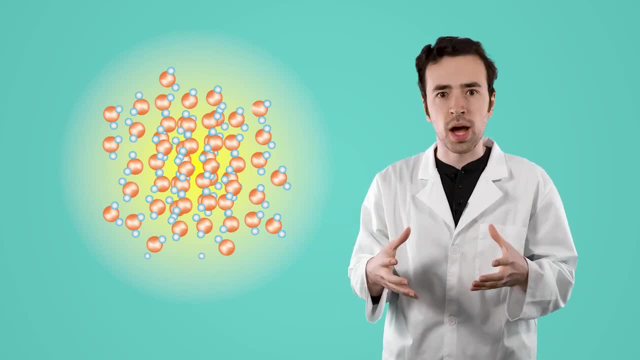 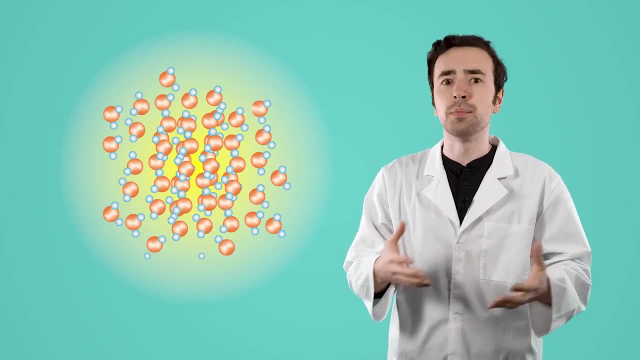 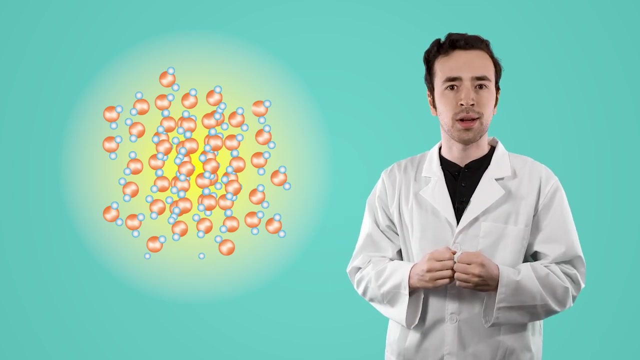 When more heat is removed, the atoms slow down even more until they're barely moving, Just kind of vibrating in place. And since they're not moving around as much, they can't really slide past each other all that well, So they end up tightly packed together. 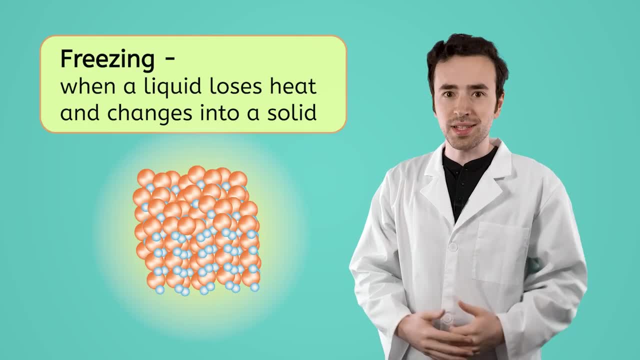 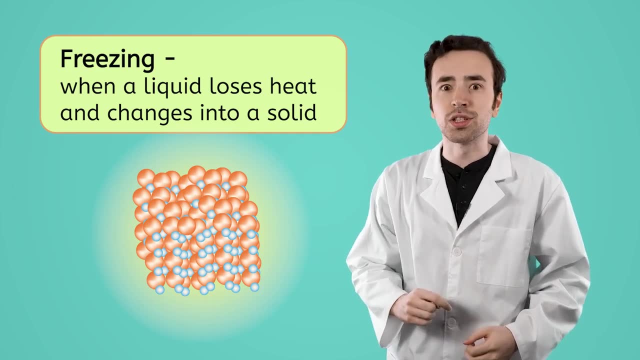 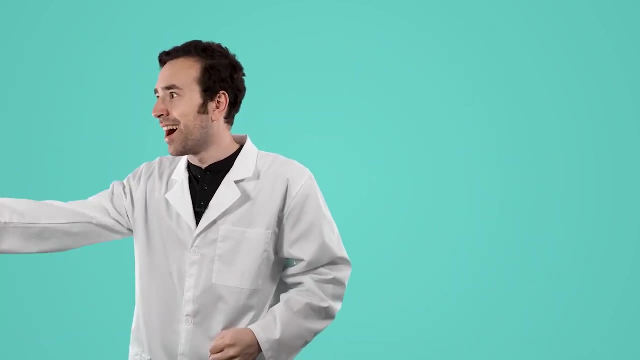 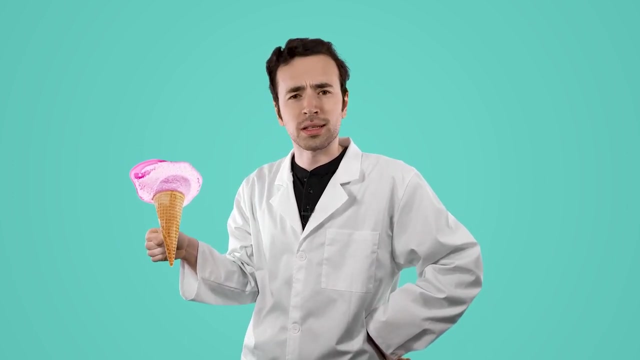 The liquid becomes a solid Freezing. And when a liquid loses heat and changes into a solid- that's the solution to the melted ice cream problem. I will just remove heat from my melted ice cream by putting it into the freezer. Well, that doesn't look quite right, does it? 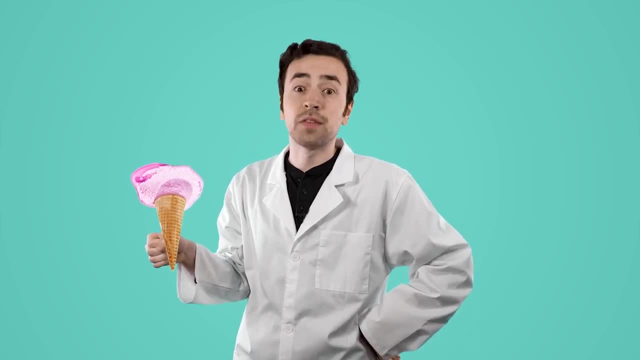 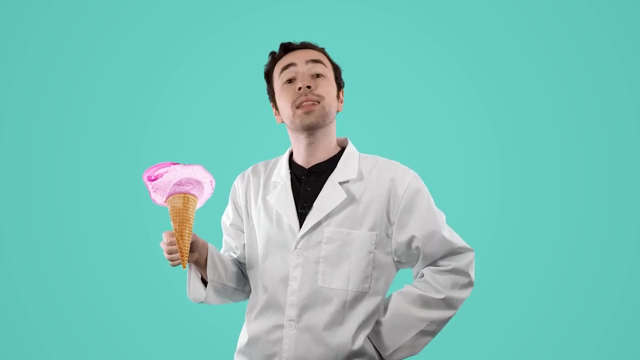 Oh, do you know what happened? Well, liquid doesn't have a definite shape, does it? So when it first melted, it lost. It lost its shape. It's ice cream scoop shape. Well, at least I can be happy knowing that I still have the same amount of ice cream. 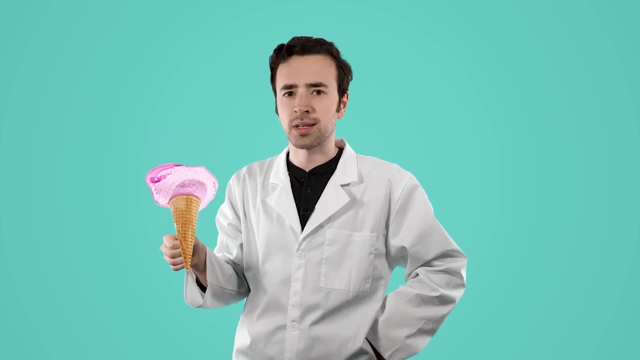 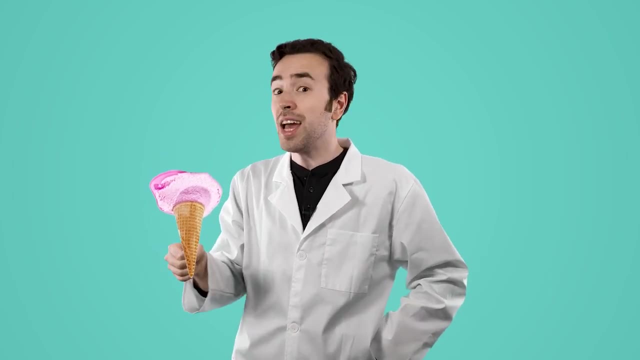 as I did before. As a matter of fact, I could melt this again, freeze it again, boil it, condense it over and over again, going through all the different state changes of matter, and I would always have the same amount of ice cream. 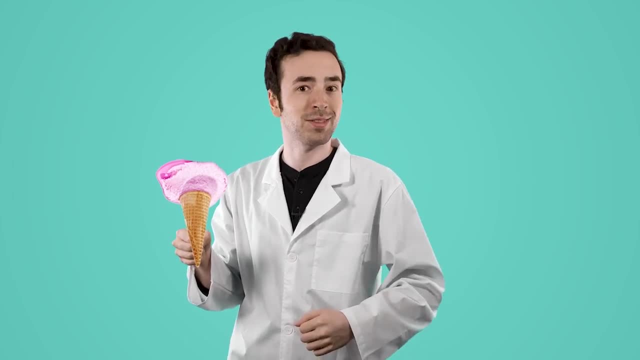 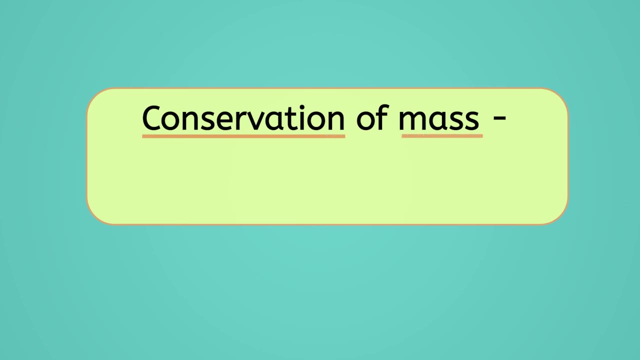 This is because of the law of conservation of mass. Conservation means to save or protect, And mass is the amount of matter in an object. So conservation of mass means that as matter changes, mass is neither created nor destroyed. The amount of matter in existence stays the same, no matter how many state changes it goes. 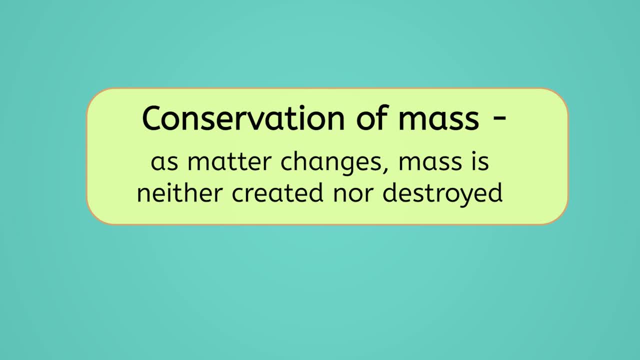 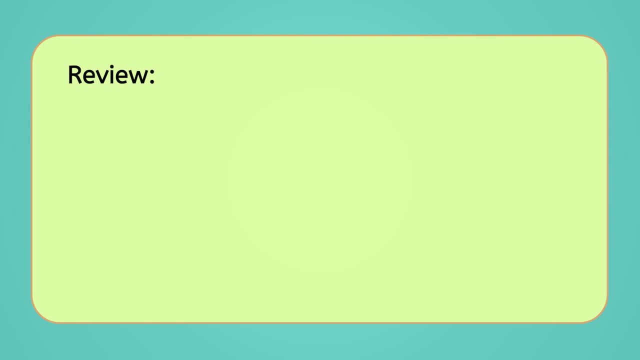 through. So my ice cream is still delicious. It's just a little lopsided now. Now that we've solved the mystery of the melting ice cream, Let's review everything we've learned today. We now know that with the addition or removal of heat, matter changes between states. 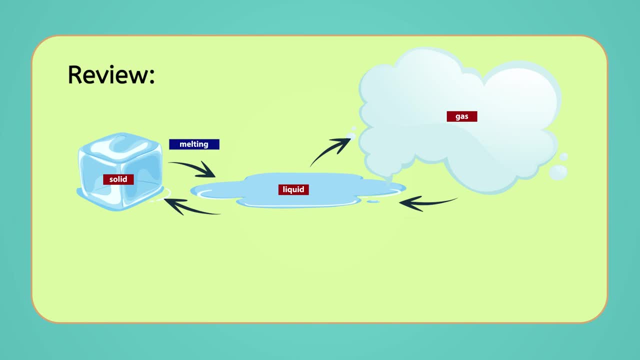 With the addition of heat, solids melt to become liquids and liquids evaporate or boil to become gases. With the removal of heat, gases condense to become liquids and liquids freeze to become solids. Throughout all of this, no matter is destroyed. 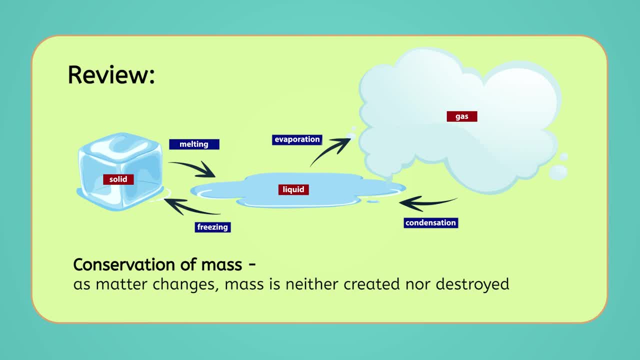 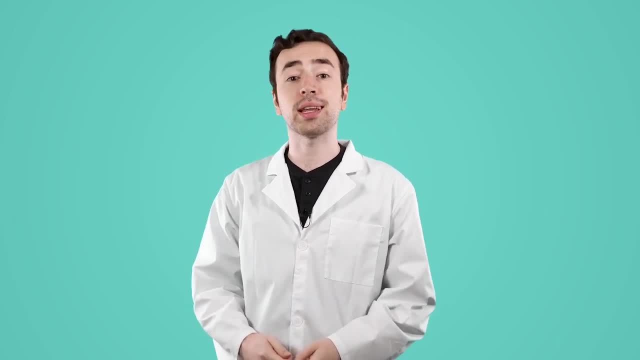 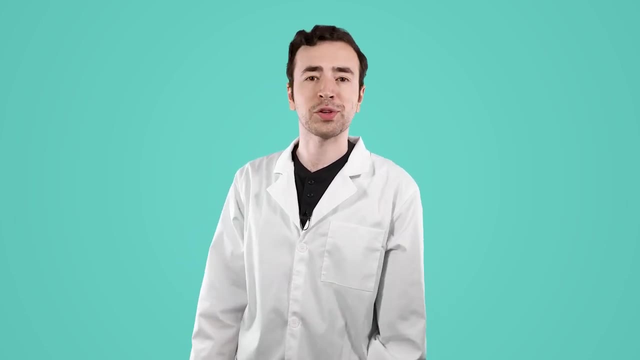 And no new matter is created due to the law of conservation of mass. To learn more about the state changes of matter, be sure to check out the practice questions and activities that go with this lesson. Well, I am off to get myself another fully intact ice cream cone.